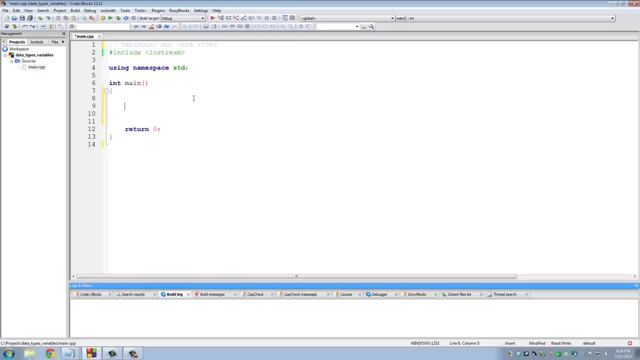 integer means it's a whole number, so it's like five, six, seven, eight, ten, one million, five million. these are whole numbers, they're not fractional numbers. they're not like 72.5 is not an integer number, okay. so anything point something is not an integer. so my age is an integer, so let's type. 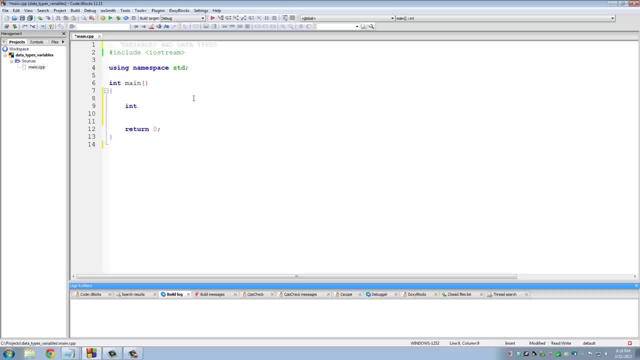 in integer. this is the type of the variable, and then i'm going to type in a name: my age, semicolon. so what happened here was i just declared my first variable and my variable is of type integer. okay, and this is the basic syntax for declaring integer. 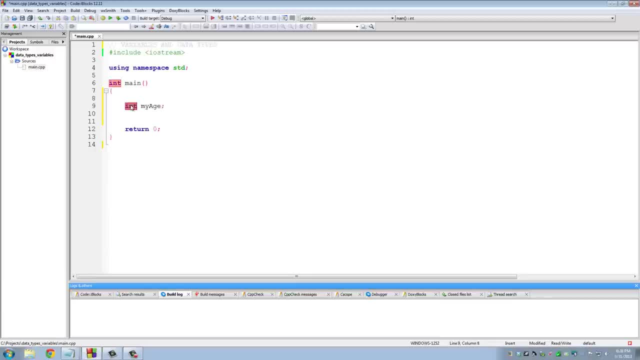 a variable that you you put in the data type. you pick a name for the variable and then you put a semicolon. okay, so let's do one more integer. let's talk about somebody else's age, their age- okay. so we just declared a variable called their age and it's of type integer. okay, so this is one of the basic data types. 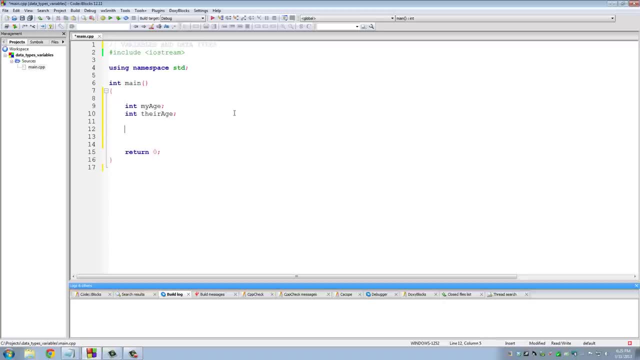 integer, integer. One of the advances in 엔는 integer. öh, okay, let's answer this with an integer. blur text text text type: double, double their money, okay. so now we have four variables, and if i said my age is 25, 25 i can store in here. if i talk about somebody else's age, i can store their age into this. 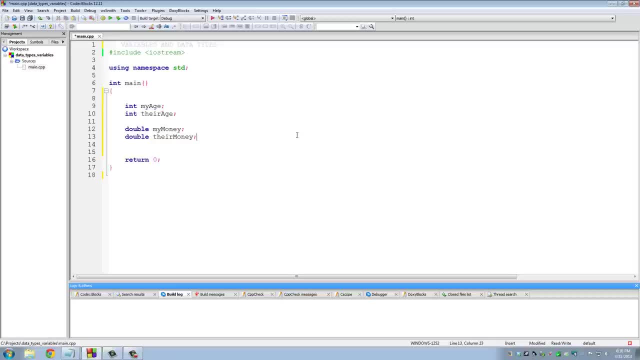 variable. so how we do that is: we use function, the function c, i, n, which is spelled like this. so let's um assign some values to these numbers, to these variables. let's initialize these variables by some numbers. we can do that right in the declaration statement. so i can start my age. 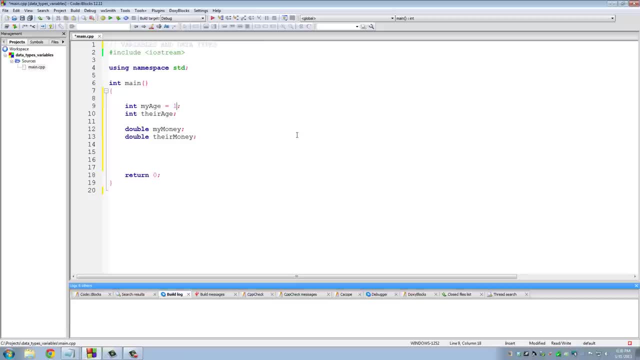 by 0 or by 15, or by 25. so this is the initial value i'm given to the variable: my age. so let's um do their age 40. okay, so let's see my money. let's say i have a 1025 dollars. and let's look at their money. 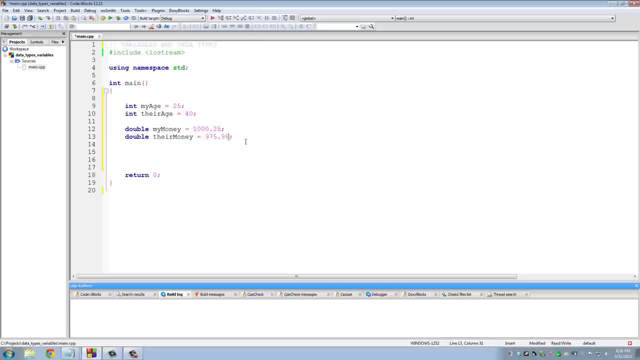 they have 975 dollars and 98 cents. okay, so be careful here. these fractional numbers can be assigned to double variables. these double variables can hold the point whatever. okay, so let's go down here and take a look at what we can print on the screen. this account, 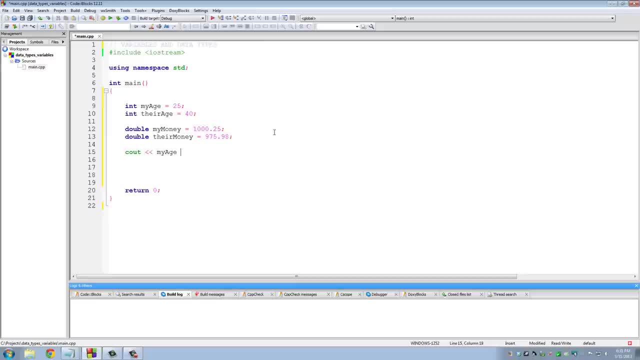 so let's go down here and take a look at what we can print on the screen. this account, my age. i'm going to put a new line. this is the new line statement. let's do count their age, okay, and then count, oops. now, by the way, c plus plus is a case sensitive language, so c out is not. 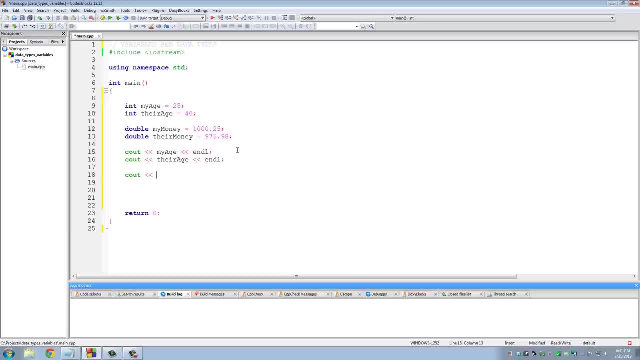 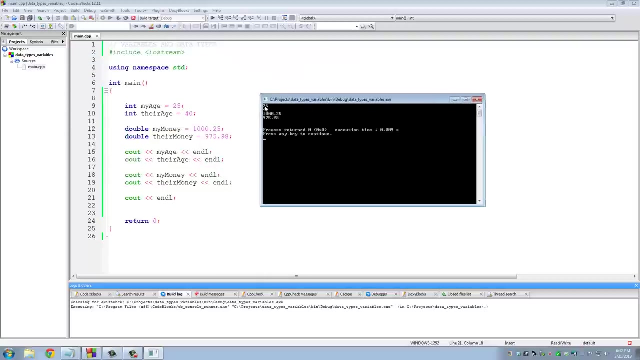 equal to c out. just remember that. okay, um, my money, let's do their money. okay, so let's, uh, just put one more new line here to keep it cleared up. let's save this program, do a build- no errors, no warnings- and let's do a run. okay, so there you go, so you get. you see the value 25, the value 40: 1000.25. 975.98. 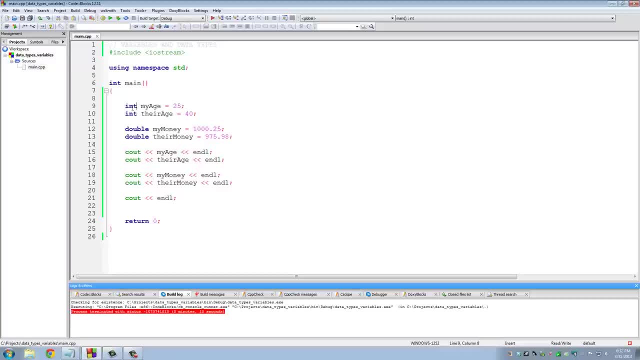 so you get, you see, the value 25, the value 40, 1000.25, 975.98. to recall, this is how we declare variables: you specify the type of the variable, you specify the name of the variable and then you can assign an initial value to that. variable. now you don't have to assign an initial variable. if you are use some driving classes, then this is important. here you use a excitable value based on your average average value. all right, now let's put that one in high estado here. just so call it down. let's get the value up, good. 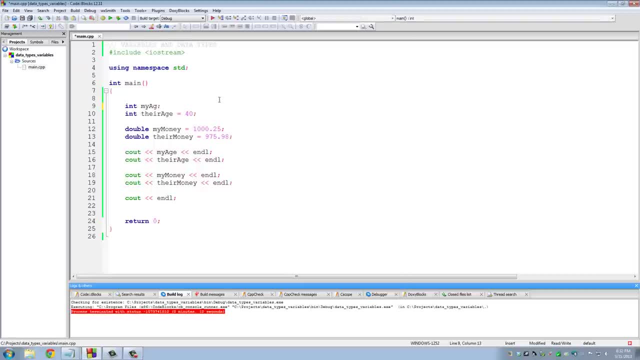 value to the variable right away. okay, you can actually do something like this: integer my age and then bottom here somewhere before you print my age, you can go: my age is equal to now. this equal to sign is actually considered an assignment sign, so it doesn't mean equal, it means assigned. so i can assign number 25. 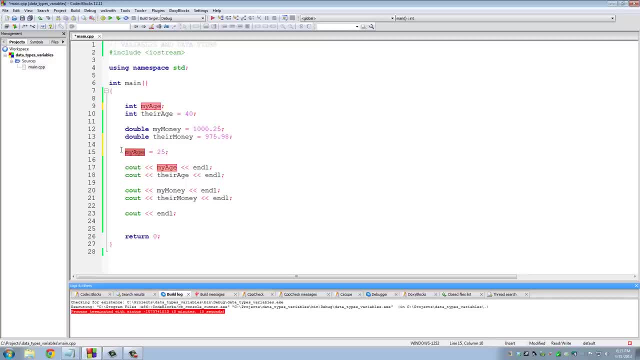 to my age. okay, so if i um save that, build it and run it, i get the same values. okay, and just uh. one more thing: if you don't initialize a variable- let's say i did not initialize my age to 25- what happens? do you think it's zero? no, it gets assigned a random variable. 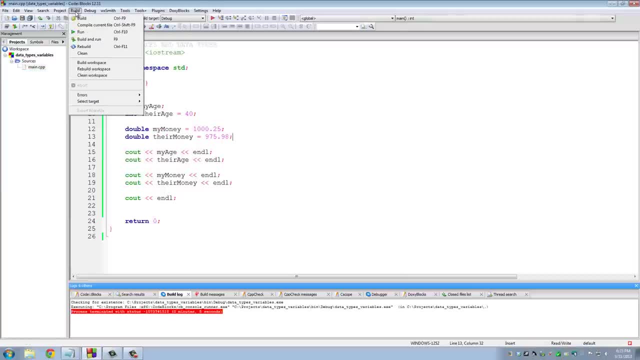 value that is going to mess up, mess you up in many ways in more complicated programs. so it is recommended that you initialize every variable that you declare. so let's do a build. you do get a warning here says: my age is used uninitialized in this function. so let's, let's. 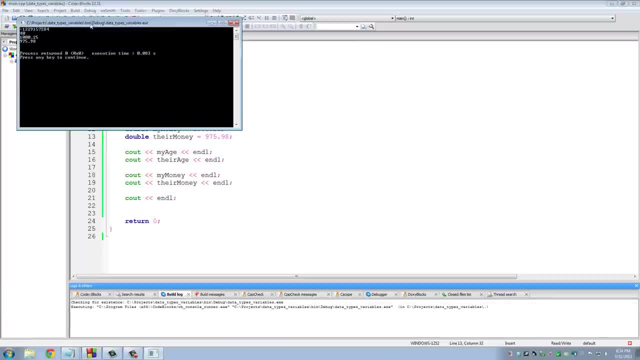 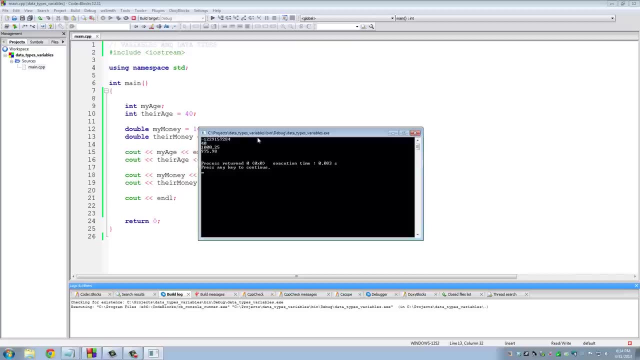 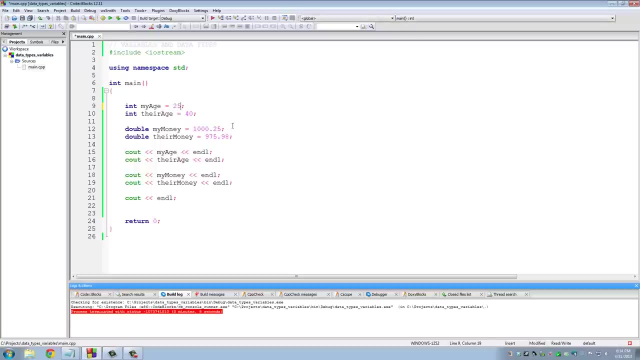 see what happens if you run this program. run the program, as you can see. it was assigned some random value that we have no idea what it is. so it's always a good thing to initialize a variable that you just declared, and obviously you don't know what everybody is. everybody's age is gonna. 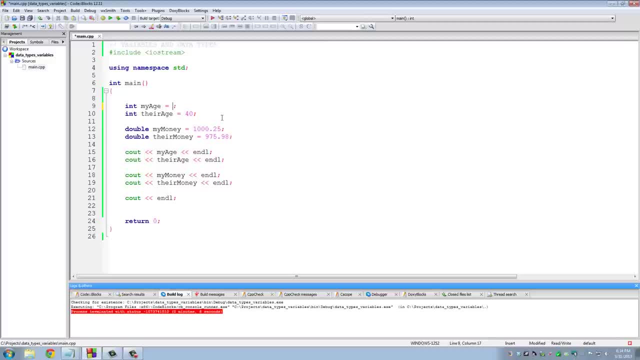 be. so it's safe to actually initialize these variables to zero, just so they have a non destructive value. you know the value of minus, blah, blah, blah. whatever we just saw on the screen was ridiculous. so after you initialize the variables here, you can reassign a brand new value to these. these guys. so their age 40, okay, and this is actually a way.